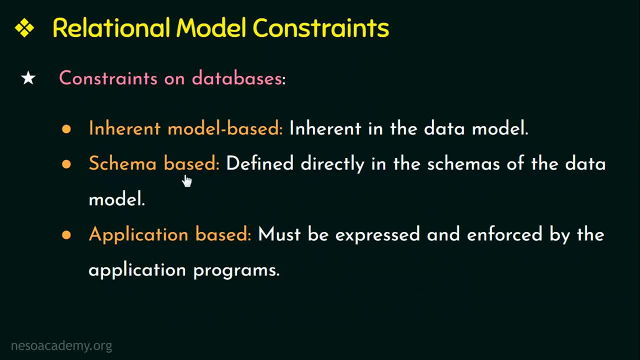 In this chapter we will be focusing mainly on the schema-based constraints. that includes domain constraints, key constraints, constraints on nulls, entity integrity constraints and referential integrity constraints. Let us see each of these constraints. So the first constraint under schema-based constraint is the domain constraints. 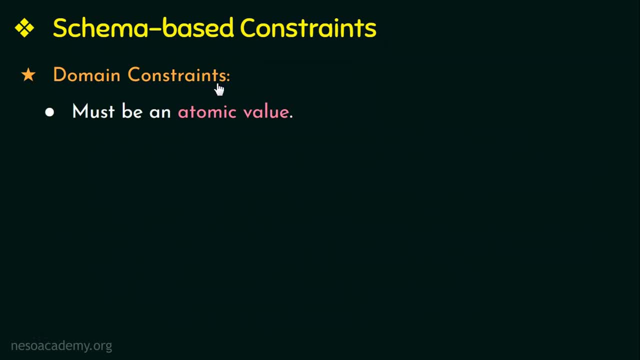 Domain constraints specifies that within each tuple or within each row, the value of each attribute has to be atomic or indivisible. Also, this constraint checks the data type of the values of each attribute. For example, in this relation, student, if I have assigned the data type of the attribute. 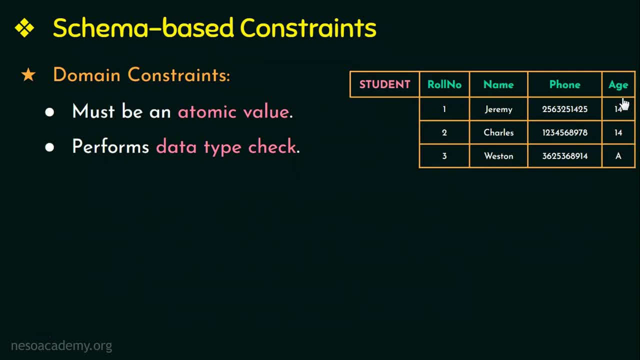 age as int, then we can't have any values in that column other than int. data type, That is, the values of the attribute age, is restricted to the data type int. So this relation violates domain constraint because we have a value in this column which 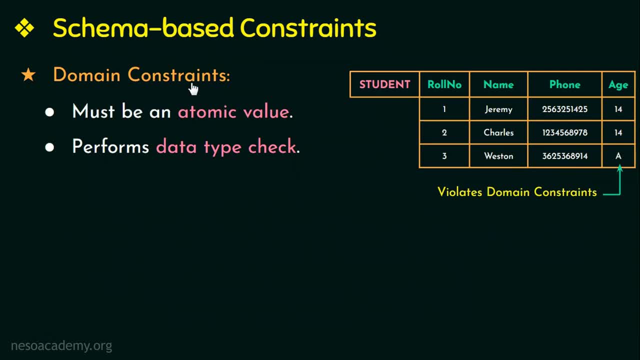 is not of int data type, So this is about domain constraints. The next type of constraint under schema-based constraints are the key constraints. We have already learned that a relation has to have a domain constraint. The next type of constraint under schema-based constraints are the key constraints. 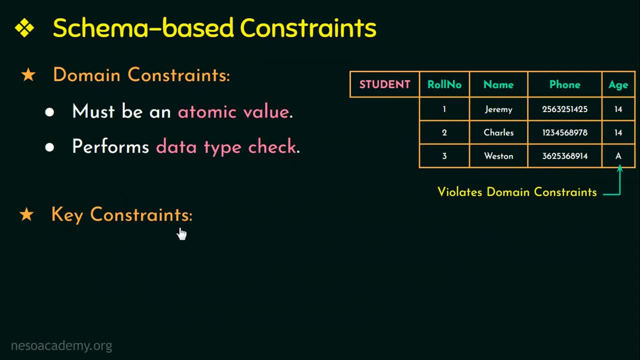 The next type of constraint under schema-based constraints is a set of tuples or rows. We know that, theoretically, relational model is based on set theory and since the elements in a set has to be unique, the tuples in a relation also have to be unique. 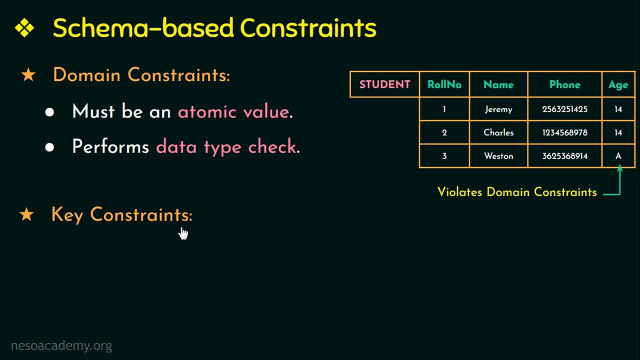 That is, you cannot have two same tuples with the same values for all the attributes. Now, when we are talking about key constraints, let us first see what a key is. We have already seen what a key attribute is in our previous video, So 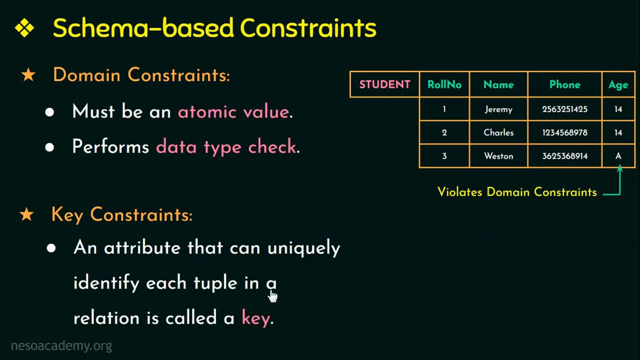 Attribute that can uniquely identify each tuple in a relation is called a key. For example, in this relation, student name cannot be a key, because we can have two or more persons with the same name. Neither can age or grade be the key, because its values are not unique. 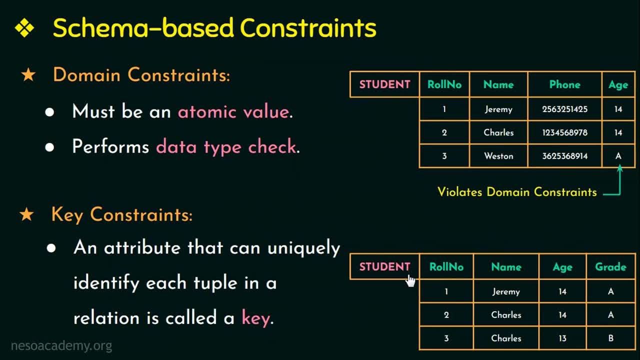 Whereas role number can be a key in this relation. student, because in a class no two students can share the same role number And hence, with this attribute, we can uniquely identify each tuple. Therefore, role number is the key in this relation. student. 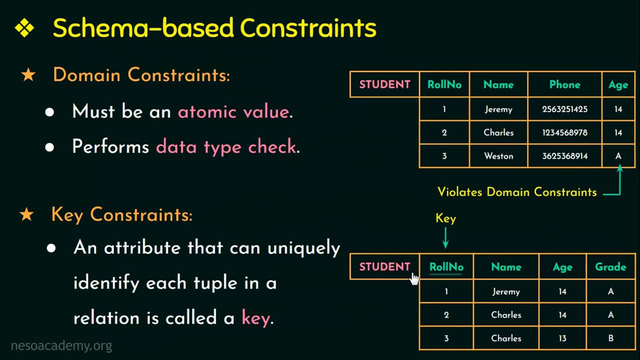 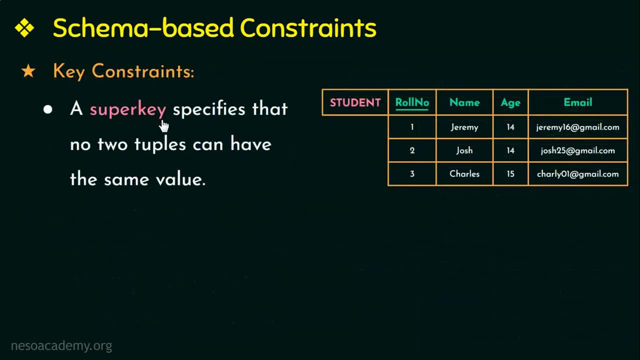 And a key in a relation is indicated or represented by an underline under the name of the key attribute. Now let us see what a super key is. A super key is a set of attributes that can help in identifying each tuple in a relation uniquely. 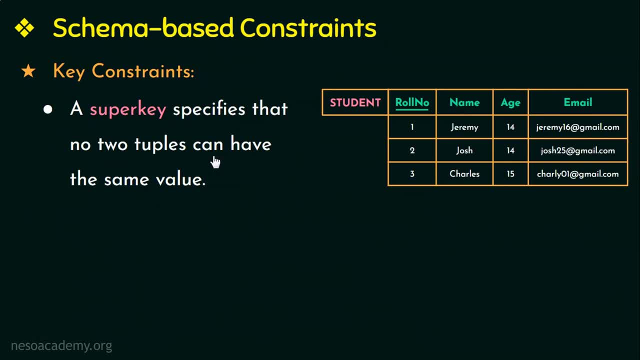 And a super key specifies that no two tuples can have the same value. That is, if role number is the super key, then we cannot have two tuples with the same value. Every relation has at least one super key by default, And that super key is the set of all attributes. 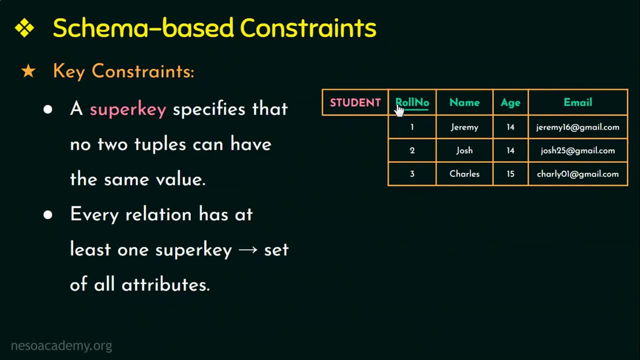 So in this relation, student, all the attributes together make a super key. That is, all these attributes together helps in identifying the tuples uniquely. So in every relation, student, all the attributes together make a super key. In every relation, by default, the set of all attributes make one super key. 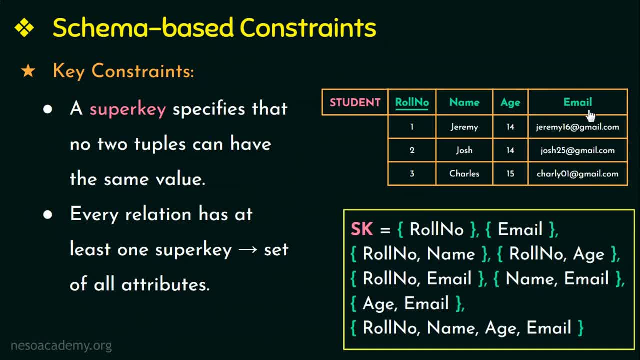 Let us identify the super keys in this relation. I have represented super keys as SK. We know that role number helps in identifying each tuple uniquely, So role number is one of the super keys. Also, no two students can have the same email id. 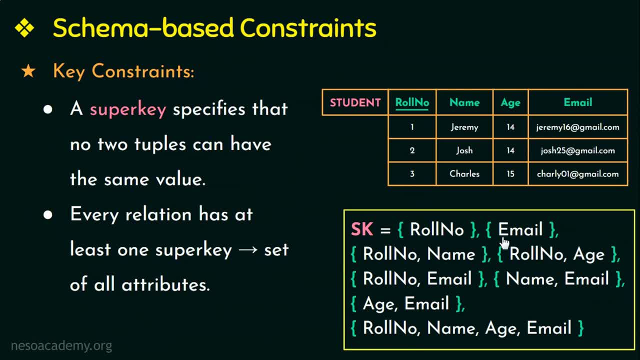 Therefore, email is a super key. Since role number and email are super keys, any set of attributes with these attributes will also be a super key. That is, the attribute name cannot identify each tuple uniquely, But when it is combined with role number, it becomes a super key. 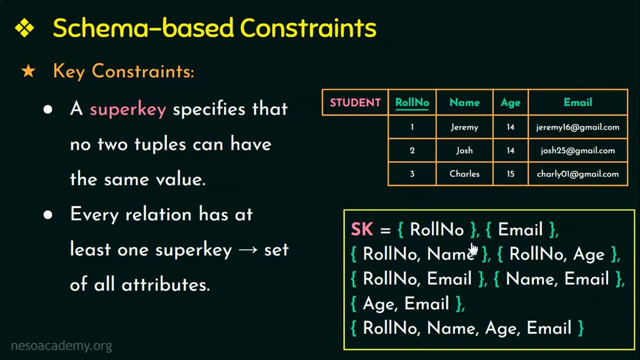 So any attributes that are combined with these super keys will also become a super key. The next super key is role, number and age. role number and email. name and email. age and email Also. role number, name and age is one super key. 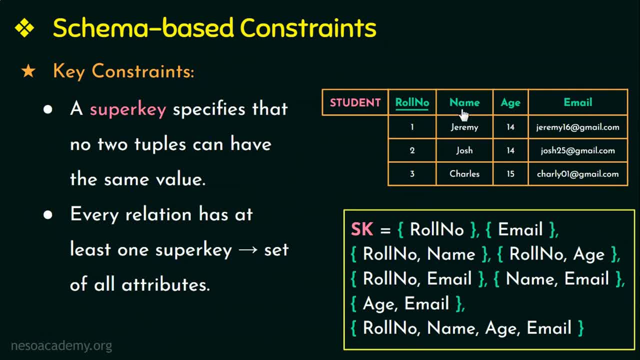 Role number, name and email is one super key. Email, name and age are super keys and age is a super key and we know by default a set of all attributes, that is, roll number, name, age and email is one super key. just remember that super key. 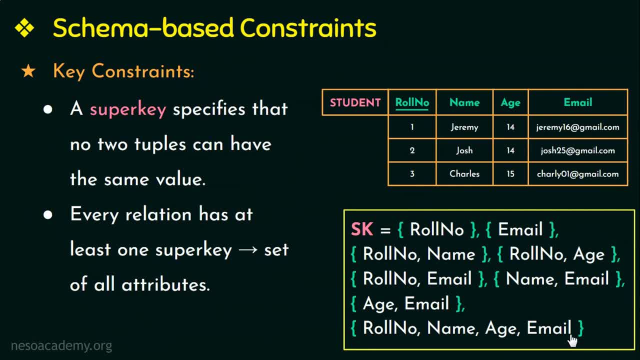 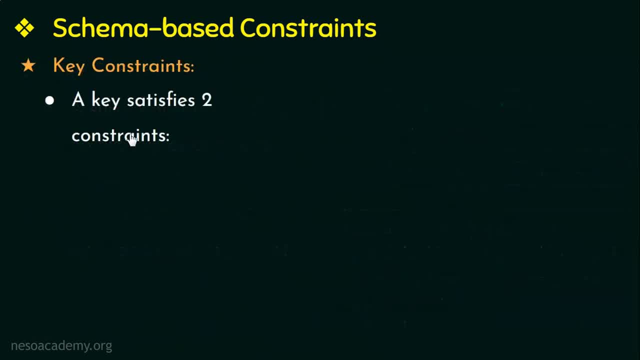 is any set of attributes that helps us to identify each tuple uniquely. so these are the super keys. in this relation, student, a key satisfies two constraints or two conditions. the first condition is two tuples cannot have identical values for all the attributes in the key. that is, in this relation, student, if this 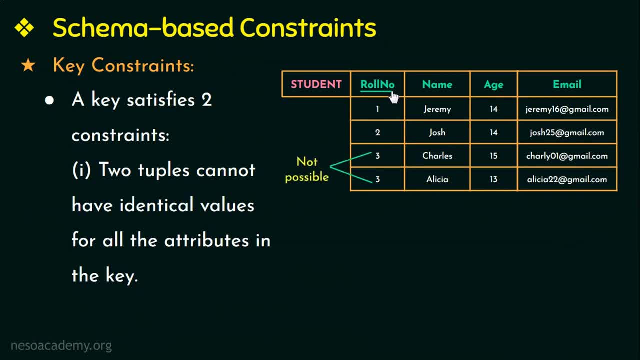 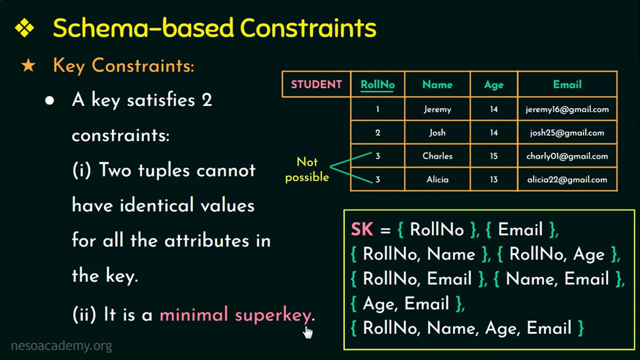 attribute- roll number has to be a key, then it cannot have two tuples with identical values. the second condition that a key should satisfy is that it has to be a minimal super key. that is the most minimum attribute to identify each tuple uniquely. we have already identified the super keys in this. 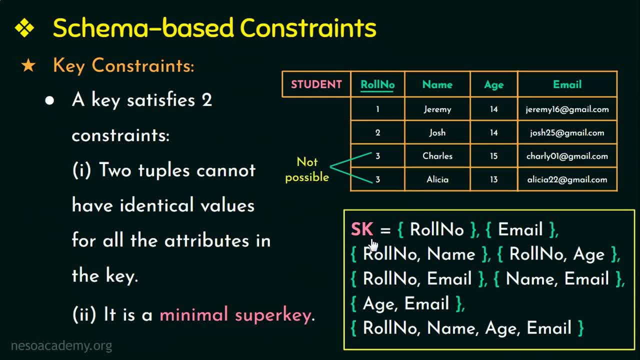 relation, and one of the conditions a key should satisfy is that it has has to be a minimal super key. Therefore, role number or email can be a key in this relation. student, This first condition is for both keys and super keys and the second condition is only for keys. Now, a relation schema can have more than one key In that. 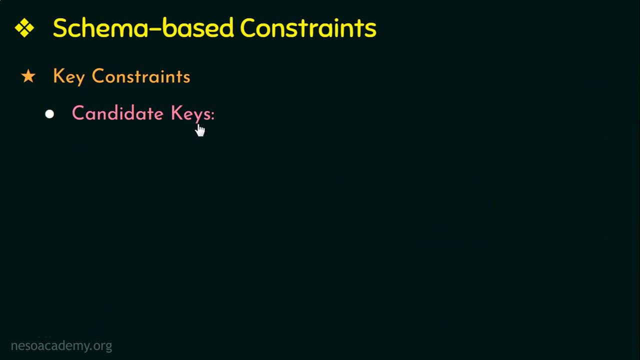 case, each of the key is called a candidate key. Again, the definitions are similar. A candidate key is a set of attributes that uniquely identify the tuples in a relation. In this student relation, we have two candidate keys. One is role number and the other candidate. 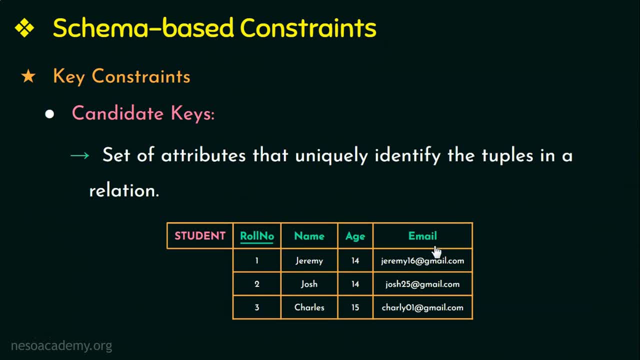 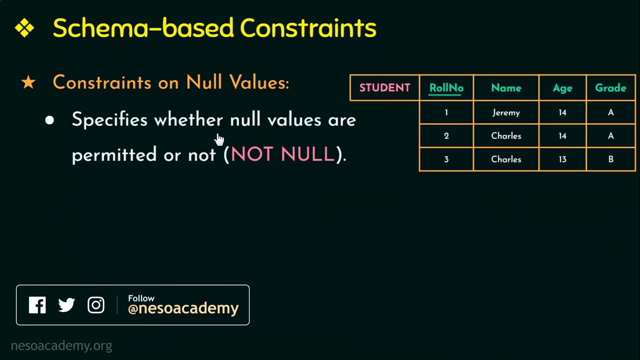 key is email. We can have any number of candidate keys in a relation, but we designate only one of the candidate keys as the primary key of that relation. Another constraint on attributes is constraints on null values. This constraint specifies whether a null value is a key or not. 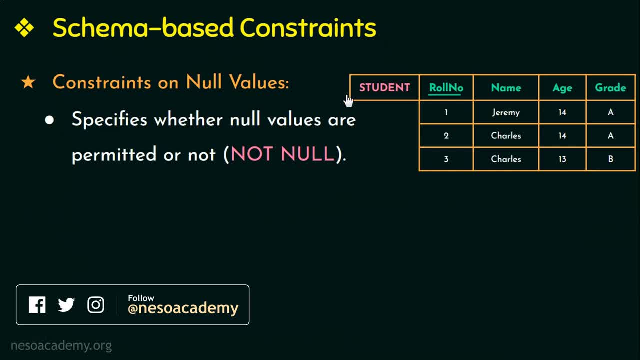 For example, in this relation, student, if every tuple in the name attribute has to have a valid value and cannot be null, then this attribute should be constrained to not null. So when I specify this constraint to any of the attributes in the relation, then the values. 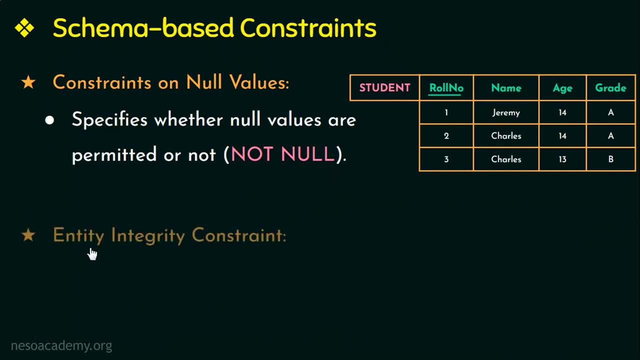 of that attribute cannot be null. The next constraint is entity integrity constraint. This constraint specifies that, or states that no primary key value can be null. And why can't it be null? Because primary key helps us to identify each tuple in the relation uniquely. And having a null value for primary 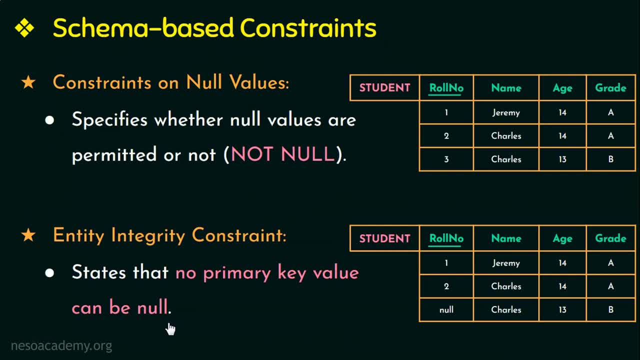 key implies that we won't be able to identify some tuples uniquely, Like, for example, this null value won't help us to identify this tuple uniquely. So therefore, primary key value cannot be null, And that is about entity integrity constraint. The next type of constraint under schema-based constraint is the referential integrity constraint. 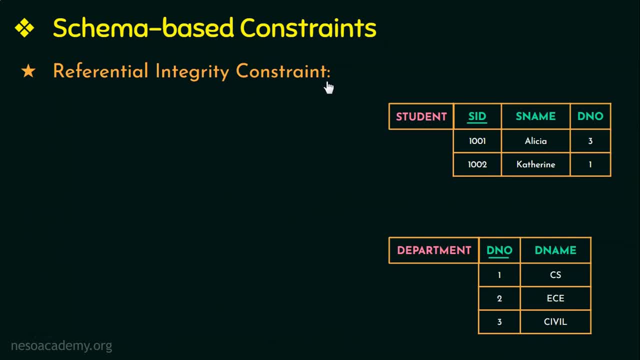 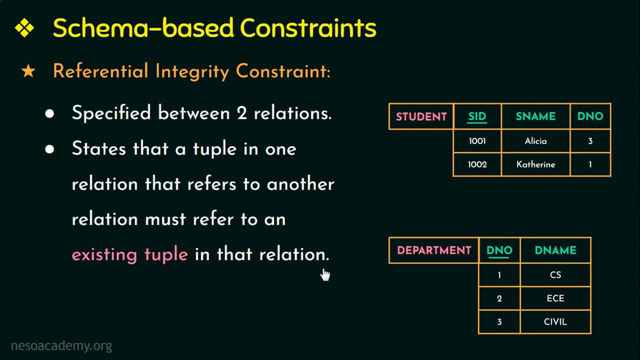 Referential Integrity Constraint states that a tuple in one relation that refers to another relation must refer to an existing tuple in the relation. Referential Integrity Constraint states that a tuple in one relation must refer to an existing tuple in the relation that relation. you will understand this definition better with the help of an. 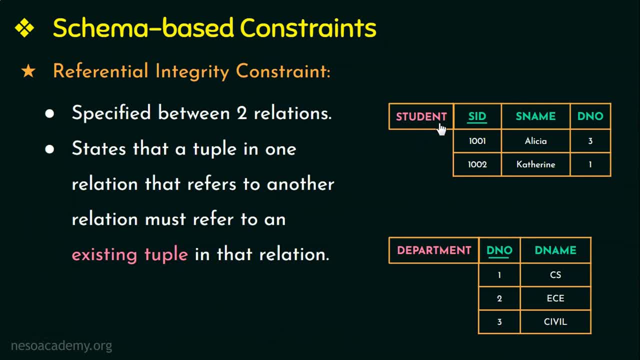 example. so here I have taken two relations. one is the student relation, with student ID as the primary key, and the department relation, with department number as its primary key. the D number of the student relation refers to the D number of the department relation. so this is the parent table and this is the 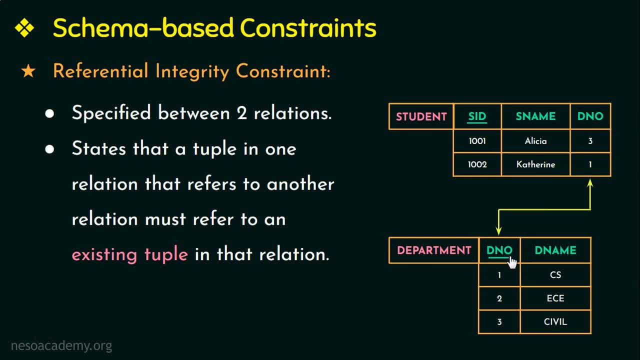 child table. since this D number refers to the D number of the department relation, the values over here in the child table should refer to the existing values in this parent table. hope you understood the definition now. referential integrity constraint states that a tuple in one relation that. 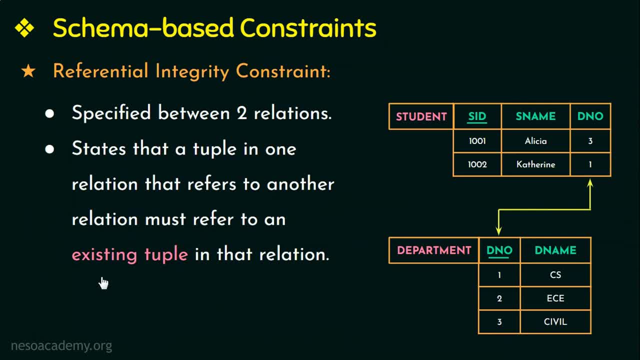 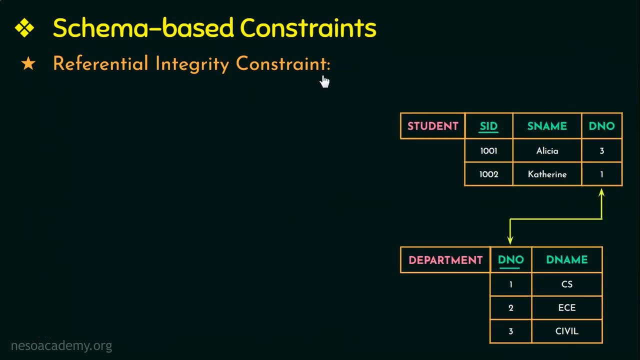 refers to another relation must refer to an existing tuple in that relation. so the attribute of one relation that refers to the primary key of another relation is called the foreign key. to understand referential integration constraints better, we need to know about foreign keys I've already defined. 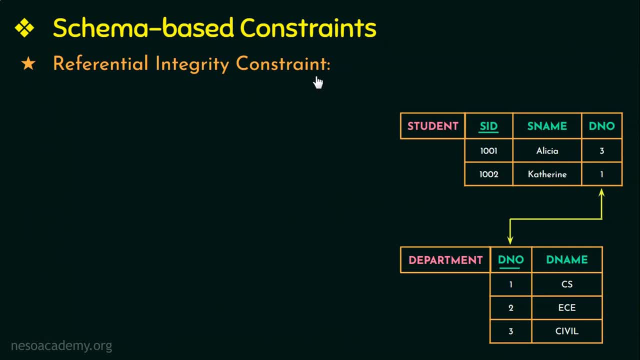 a foreign key. it is a set of attributes in a relation that refers to the primary key of another relation. a foreign key must satisfy the following conditions. the first one is it has to be of the same domain as the attribute it refers to. we know that D number is the foreign key as it refers to the primary key of.